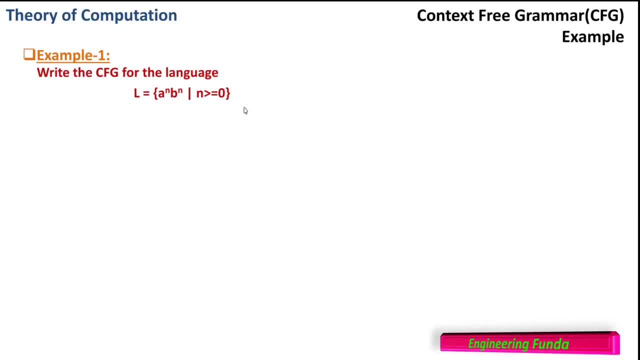 language. Once we understand this language and its grammar, then we will be able to define many other languages. We will be able to define many other languages. We will be able to define many other languages. Let us start understanding this, My dear friends. in the case of regular 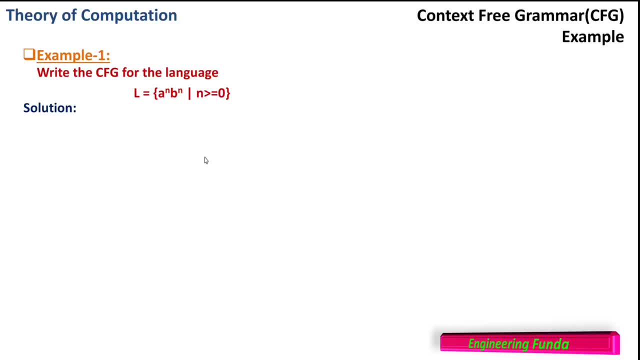 language. we have started understanding that by using the language set. The same. we are going to do it here, my dear friends. The language set consists of these words. We are saying that n is greater than or equal to 0. That means the smallest value of n is 0.. 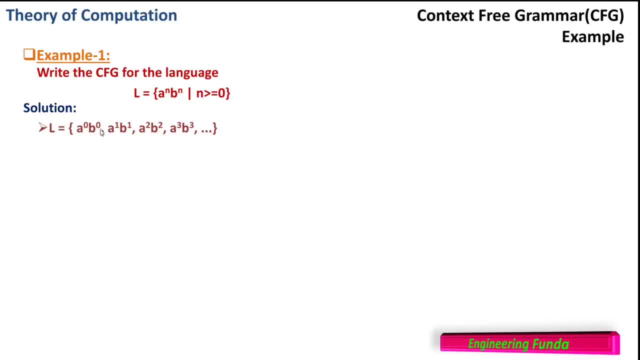 So the first word is n, The second word is n, The third word is n, The fourth word is 7.. So the third word will be a raised to 0, b raised to 0.. Now, what does this power? 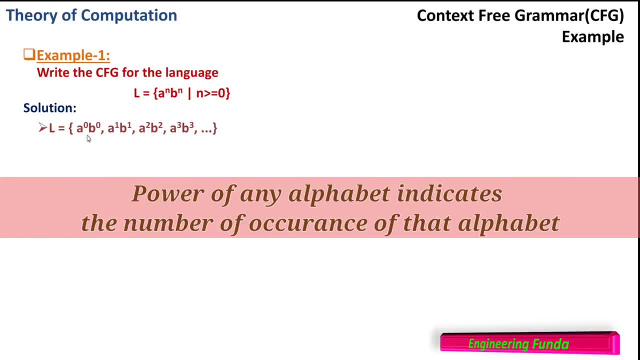 here indicate my dear friends, Power. here indicates the number of occurrences of that particular alphabet. If I say a raised to 0, that means the number of occurrences of a is 0. That means actually a is not present, which is an empty string. So empty string. is null. Same way b raised to 0. So b raised to 0.. E is not present, So empty string is null. It is equal to 0.. Now what does this beaquile me to say as an empty string String? 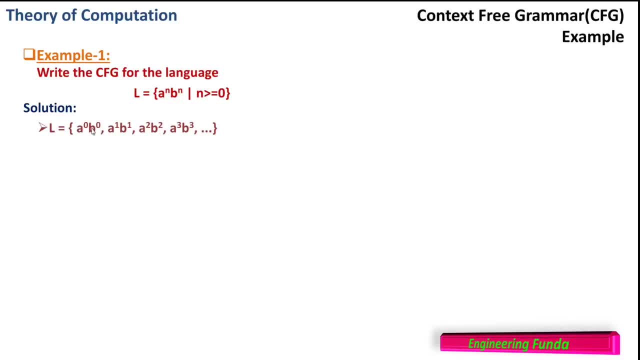 which is non-existent. So empty string will be 0.. So if I say letter n, it is also null. So B raised to 0 is also null and null followed by null will be the null. So first string that is there in this L is null. 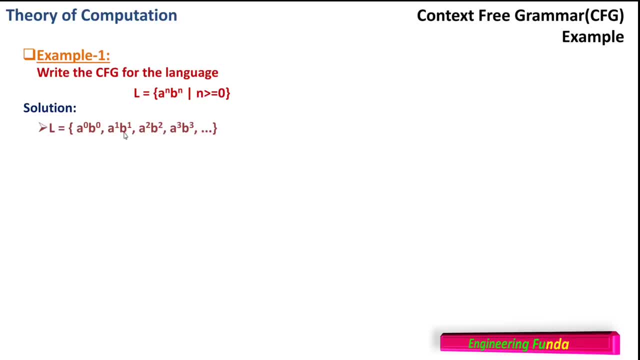 Same way, A raised to 1, B raised to 1 will be AB. simply A raised to 2, B raised to 2 will be AABB. This is how we can write it. The first is a null string, epsilon. Second is AB. 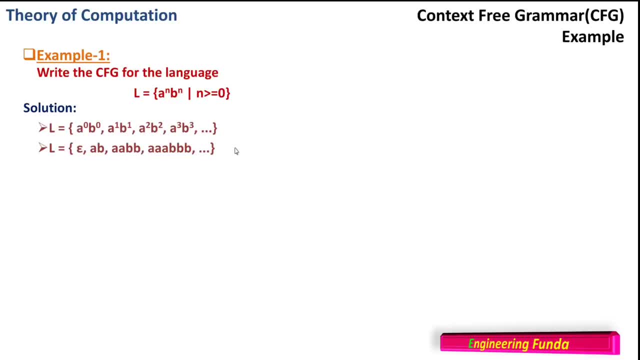 Then you have AAWB and 888BB And so on. Here we have to start observing the language from the minimum length string And try to find the pattern in which the string gets built up. The same approach that we have taken for the regular language and regular grammar. 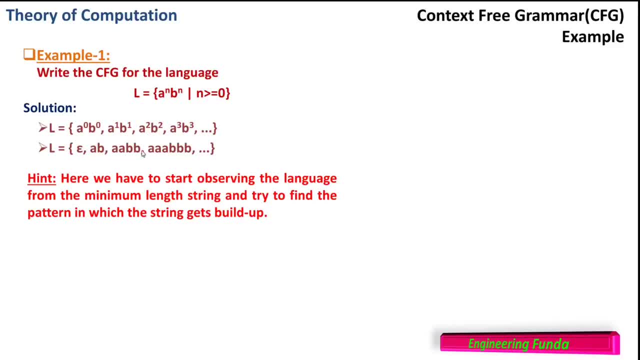 That is, we are trying to observe the pattern how it is getting generated. First we start from the minimum length string. So here This minimum length string is epsilon or the null string. That means the minimum length string here is epsilon, which is having the length 0.. 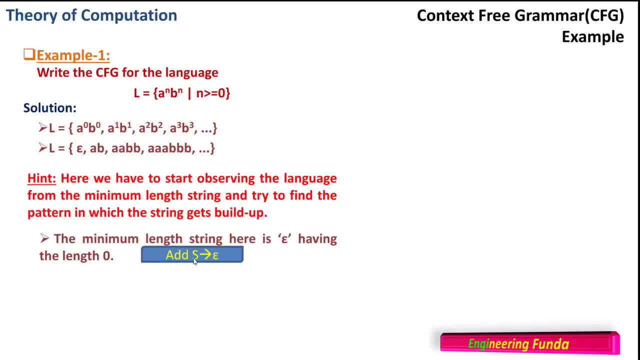 If this is the case, then we have to add the production S tends to epsilon to my grammar, Where S is my starting state. Now, why is this required? Because the epsilon can only be generated From the language by traversing from the starting symbol, or any word can be generated by traversing from the starting symbol. 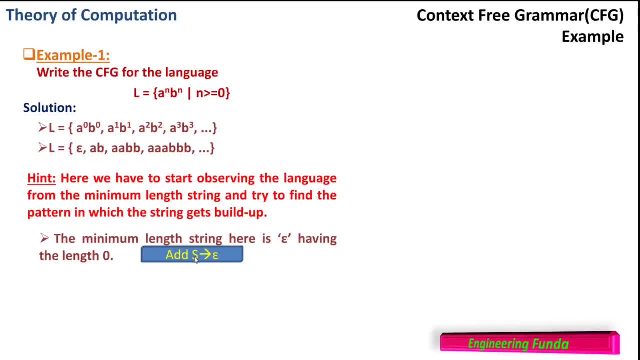 Now if epsilon belongs to my language then we have to have the production. S tends to epsilon in my in the grammar. But epsilon on the null string will not help us in identifying any pattern Because epsilon is a null string. we cannot see any pattern in the epsilon. 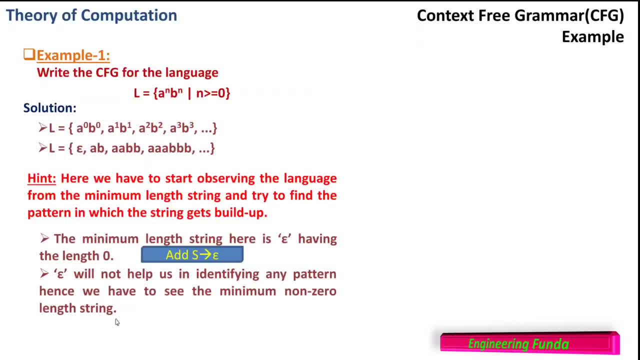 Hence we have to see the minimum non-zero length string. The minimum non-zero length string in the language is AB. The first word, the first non-zero length word that is there in the language is AB. So we have to keep this AB in the focus. 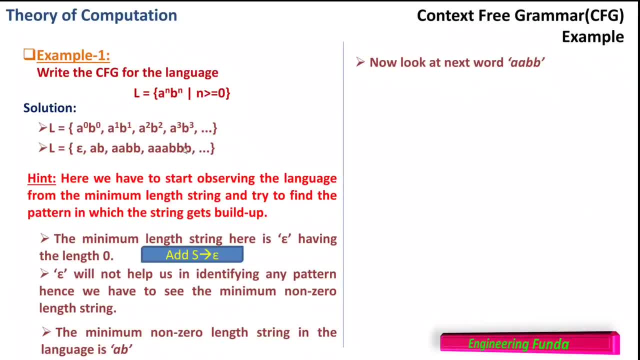 Now let us see the minimum non-zero length string. Let us see the minimum non-zero length string in the language. Now let us look at the next word, which is AABB. The second word, or the third word, is AAWB. The word AAWB have AB as a part in it. 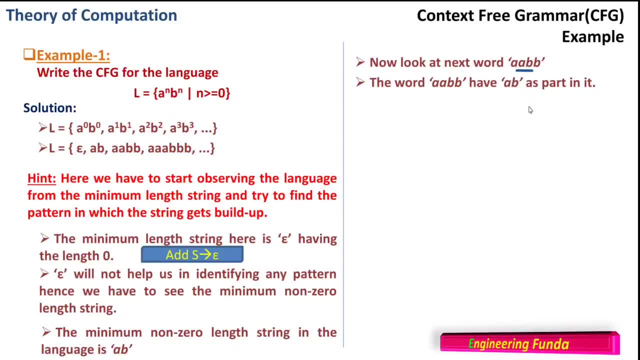 If we see the center part, we have AAWB as the word And in that AAWB we have center as AB. So the minimum non-zero length word is a part of Of the next word. This gives me a hint that, my dear friends, 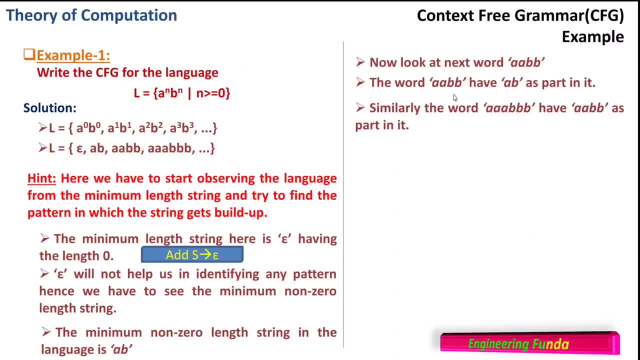 using AB, we can generate AAWB. Similarly, the word AAABB have AAWB as a part in it. Hence, to generate a word using a grammar, we make use of a variable or a non-terminal, And we need to use a variable or a non-terminal. 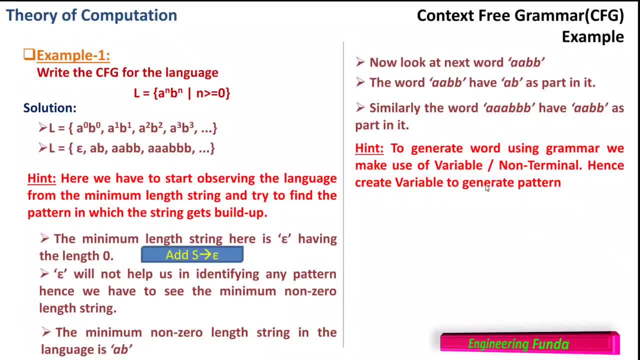 So we need to create this variable to generate the pattern. Let us see how we can do that. The minimum non-zero word, non-zero length word generated in the language is AB. So first I need to add this: production S tends to AB to my grammar. 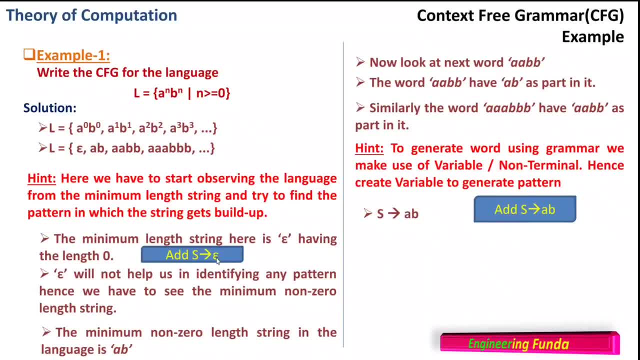 Now my grammar have two productions: First is S tends to epsilon And second is S tends to, Because we are trying to generate the words. And to generate a word we need to first understand the pattern And in the pattern we need to find out the minimum non-zero length word that can be used repeatedly. 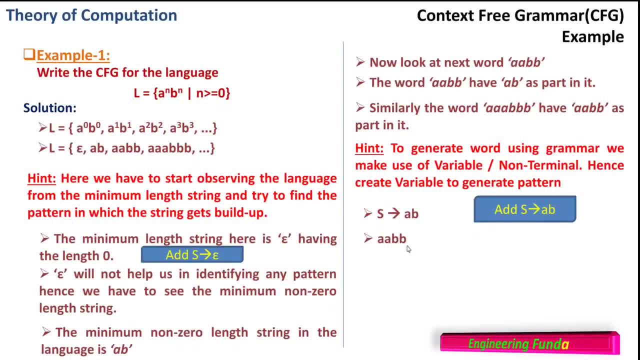 Now the next word is AABB. So here I can see that I have this grammar: S tends to AB. Now this AB can be replaced by S, So this can become ASB, Now ASB. So if I have this ASB in my grammar, then I can generate AABB. 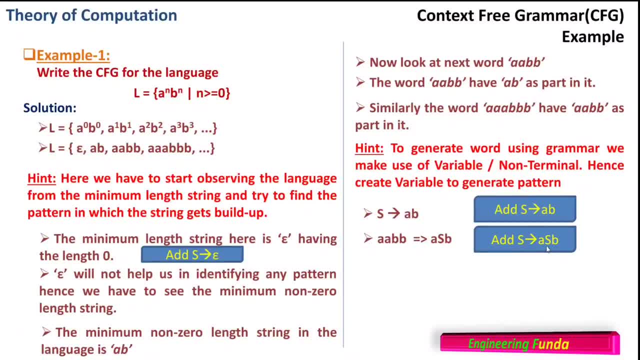 So what I say is: add this production S tends to ASB to the grammar. So my grammar now have three productions. Let us look at the another word, That is AAA, BBB. Now AAA, BBB. Again. I have this AB. 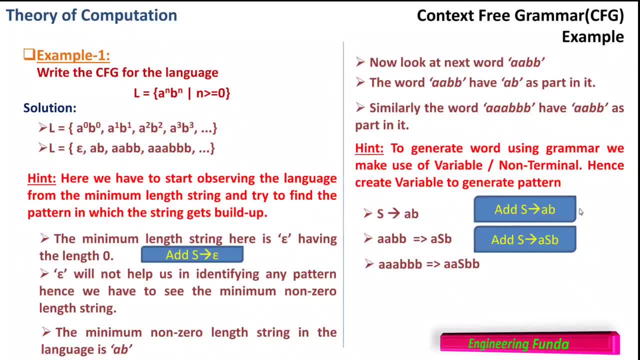 So I am replacing it with S, As per the first production that is added, Because I want to generate this. So what I am doing is I am going in the reverse manner. Now, one thing that I can do is I can add this AASBB to my production group. 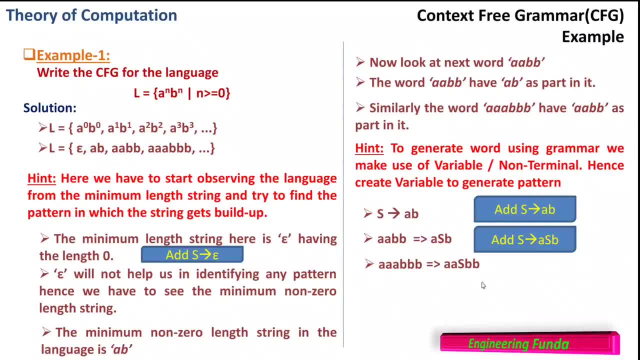 But there is one more observation here, that is AASB. I can generate from the grammar. That means I can use this S tends to ASB and generate this AASB. So this AASB can be replaced with S. So I have this. 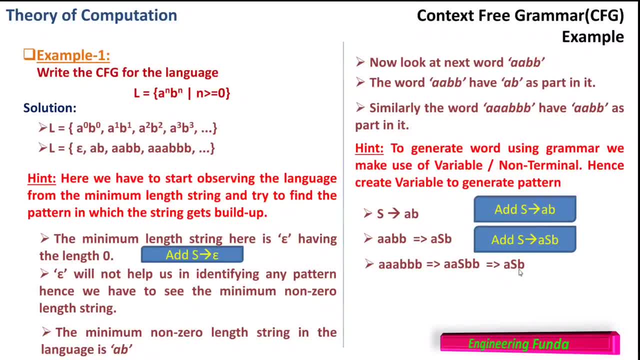 What I am trying to do is I am trying to minimize this. Now, this is AASB, So AASB I cannot generate, But this already can be generated. This already exists in my productions. That means I have the production rule. S tends to ASB.